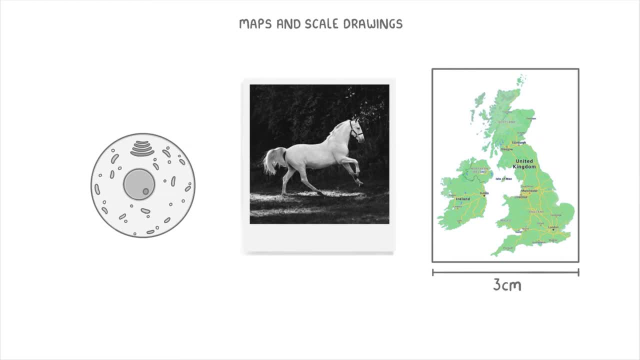 or larger than the real things, so that we can show them neatly on the space of the screen. However, the important thing to notice is that the images are to scale, which means that all of the proportions are correct, For example, the horse's height relative to. 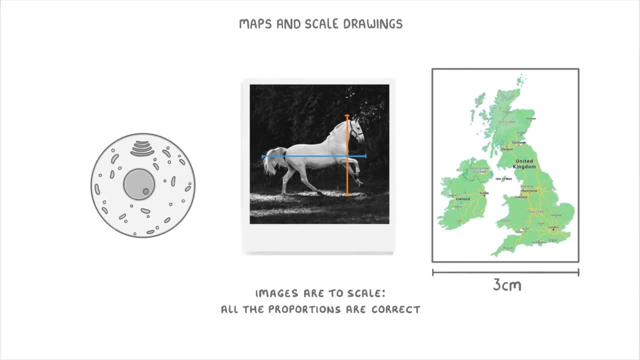 its length is correct. There's a bit of confusion around what we call images like this, because it depends on what type of image we have. If we have a photo, then we just call it a photo, because they should always be to scale When we have a drawing. that's to scale, though we call. 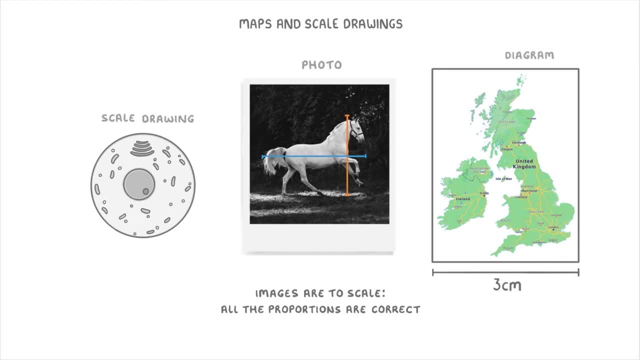 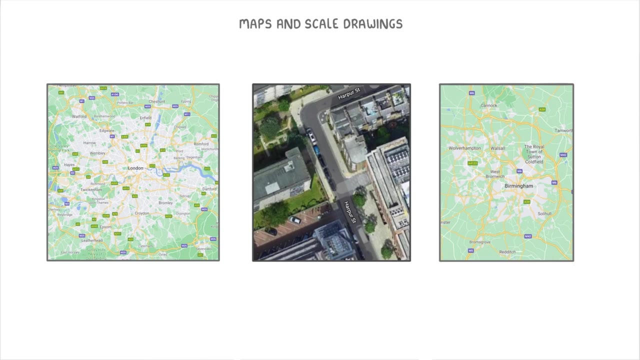 it a scale-wise, And when we have a diagram that's to scale, we call it a scale-diagram, Although in the special case of a map, we can also just call it a map as well. Now, something else that all scale diagrams or maps should have is some kind of scale. 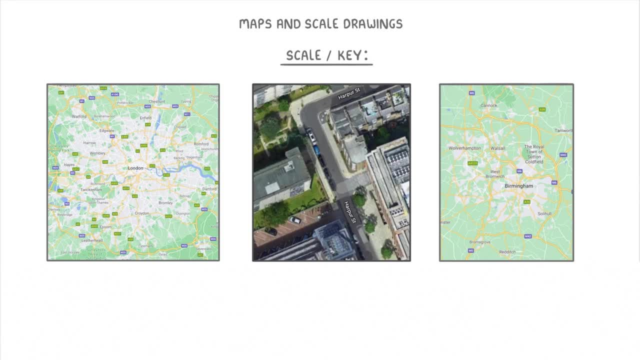 or key which allows you to work out the real-life distances that the images represent. There's a few different ways they can do this, but the main ones are these three. This first type is the easiest to work with, and in this case it just means that every 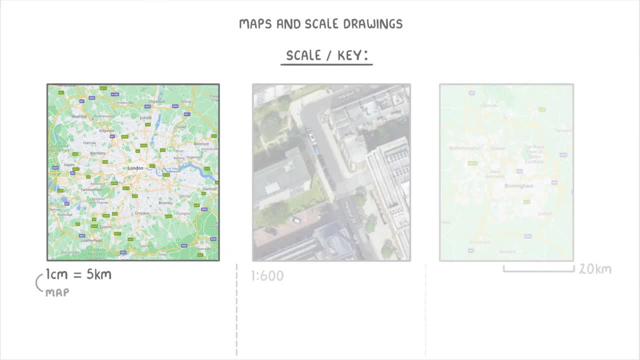 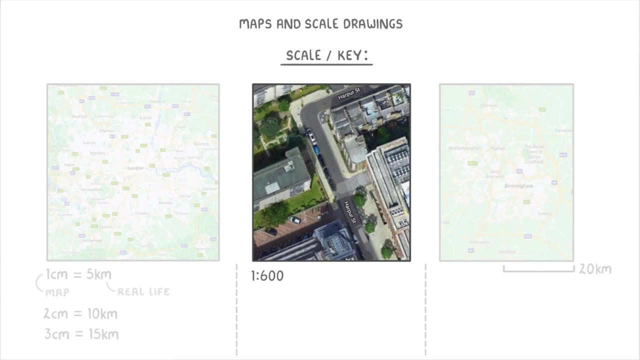 one centimetre on your map or drawing represents 5 kilometres in real life. So 2 centimetres would represent 10 kilometres, 3 centimetres would represent 15 kilometres, and so on. This second one- 1 to 600, is basically a ratio and means that everything on the image 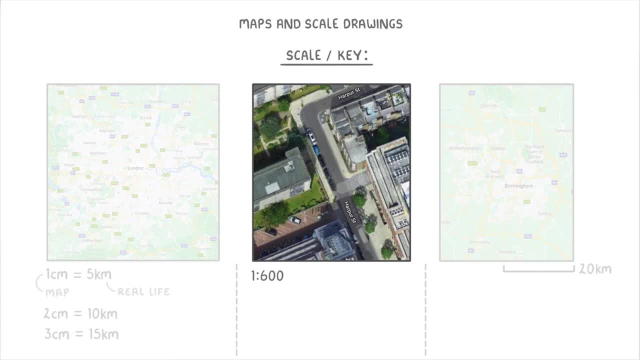 is 600 times smaller than the real thing, Or enough. In other words, every one centimetre on the image would be 600 centimetres in real life, So we could rewrite it as 1 centimetre equals 600 centimetres, or even 1 centimetre equals. 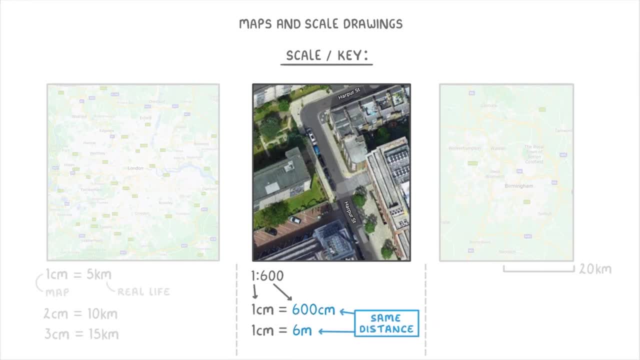 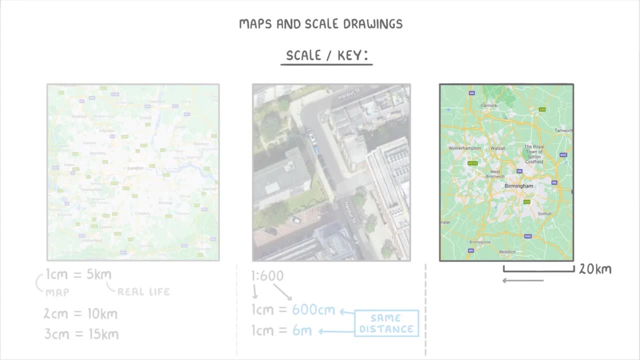 6 metres, because 600 centimetres and 6 metres are the same distance. This last type is the trickiest of the three, but just means that this distance here represents 20 kilometres. So what we normally do is measure the line with a ruler. 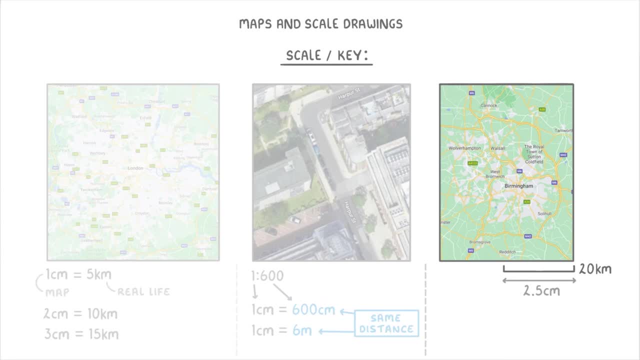 which in this case would be 2.5 centimetres. and then we know that every 2.5 centimetres represents 20 kilometres, which is a much easier scale to use- And if you wanted, you could make it even easier by dividing both sides by 2.5, to find. 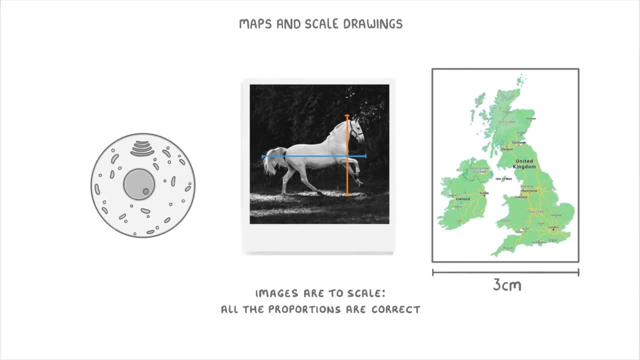 its length is correct. There's a bit of confusion around what we call images like this, because it depends on what type of image we have. If we have a photo, then we just call it a photo, because they should always be to scale When we have a drawing. that's to scale, though we call. 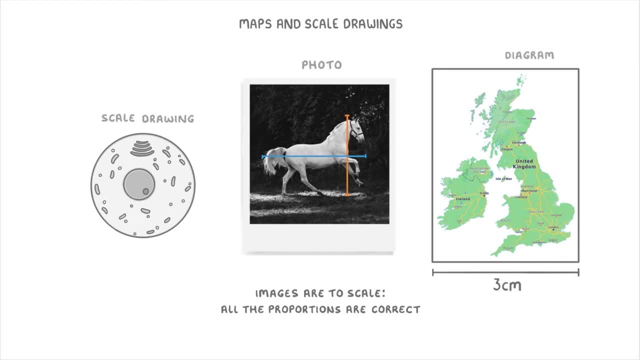 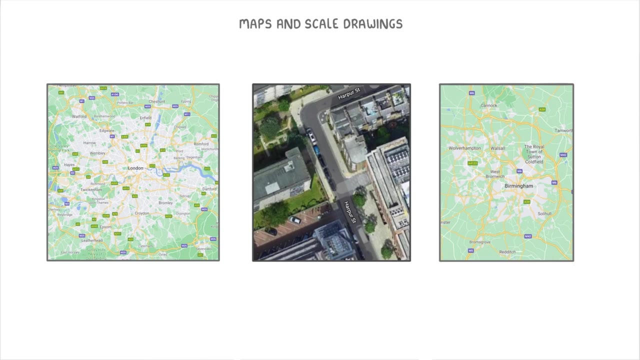 it a scale-wise, And when we have a diagram that's to scale, we call it a scale-diagram, Although in the special case of a map, we can also just call it a map as well. Now, something else that all scale diagrams or maps should have is some kind of scale. 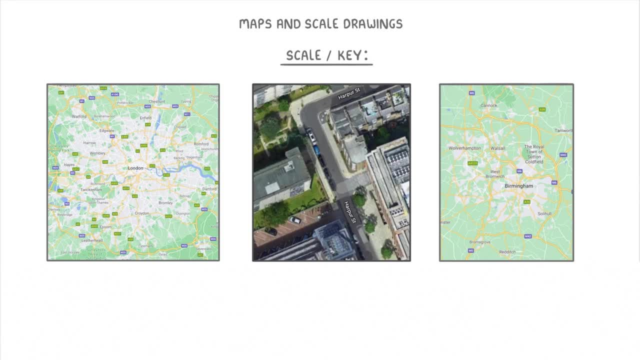 or key which allows you to work out the real-life distances that the images represent. There's a few different ways they can do this, but the main ones are these three. This first type is the easiest to work with, and in this case it just means that every 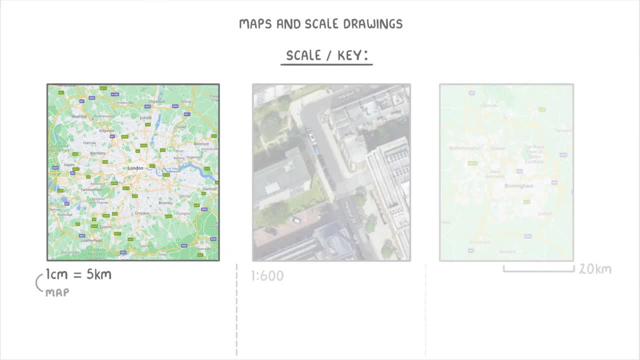 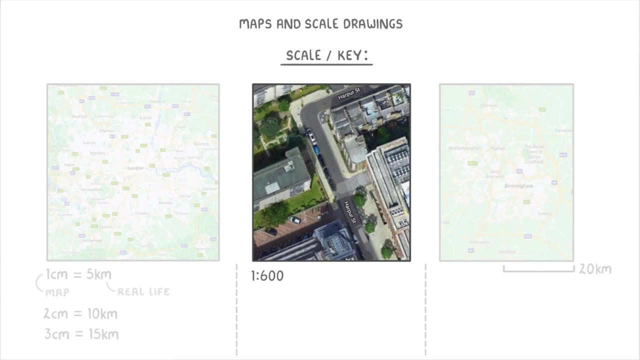 one centimetre on your map or drawing represents 5 kilometres in real life. So 2 centimetres would represent 10 kilometres, 3 centimetres would represent 15 kilometres, and so on. This second one- 1 to 600, is basically a ratio and means that everything on the image 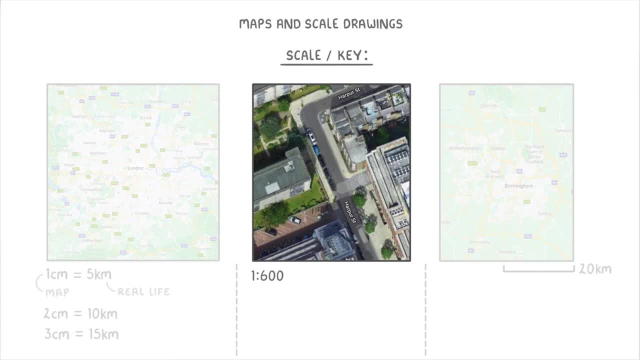 is 600 times smaller than the real thing, Or enough. In other words, every one centimetre on the image would be 600 centimetres in real life, So we could rewrite it as 1 centimetre equals 600 centimetres, or even 1 centimetre equals. 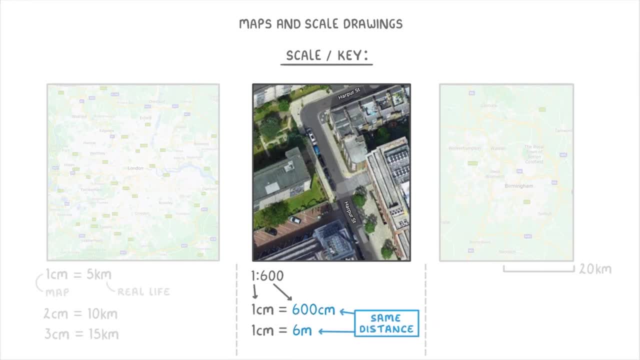 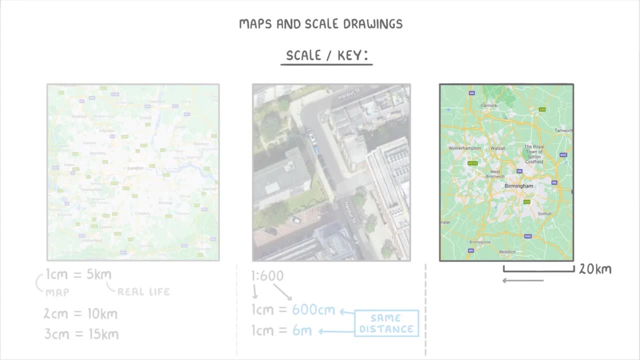 6 metres, because 600 centimetres and 6 metres are the same distance. This last type is the trickiest of the three, but just means that this distance here represents 20 kilometres. So what we normally do is measure the line with a ruler. 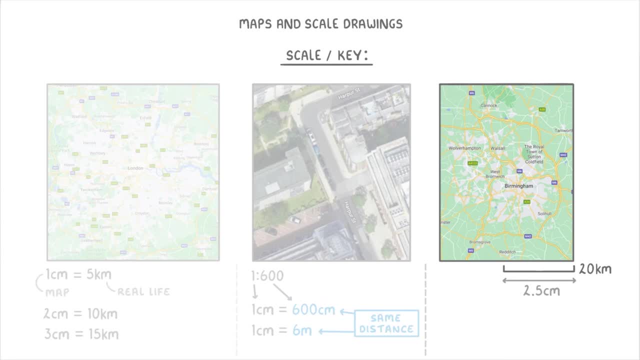 which in this case would be 2.5 centimetres. and then we know that every 2.5 centimetres represents 20 kilometres, which is a much easier scale to use- And if you wanted, you could make it even easier by dividing both sides by 2.5, to find. 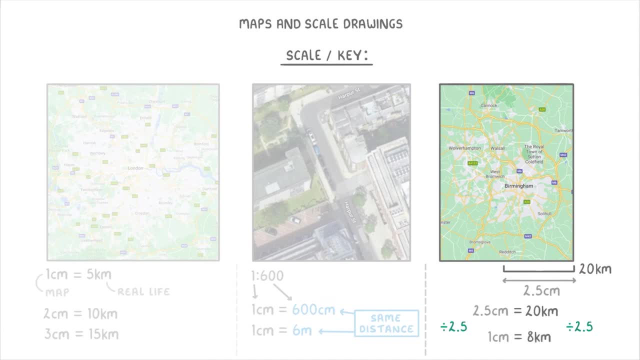 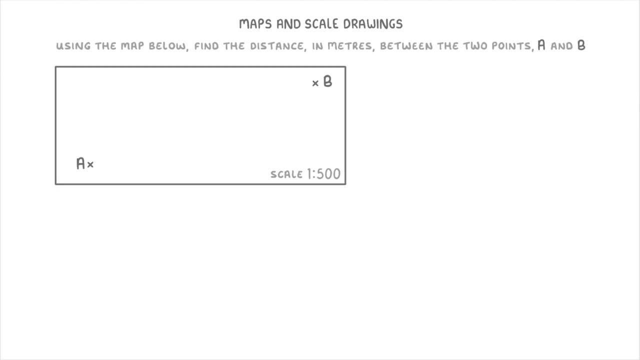 that 1 centimetre represents 8 kilometres. Now that we've covered the basics, let's have a go at a couple of exam questions. So in this question, we're being asked to use the following formulae: So in this question, we're being asked to use the following formulae: 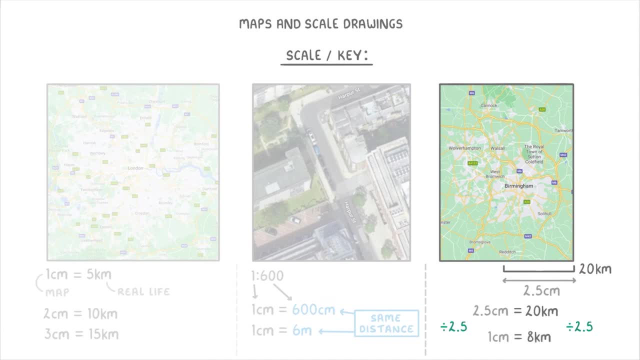 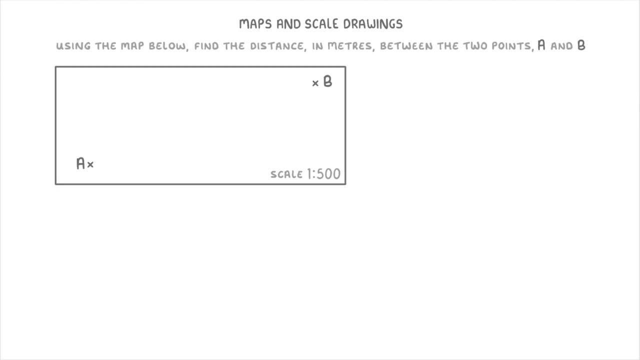 that 1 centimetre represents 8 kilometres. Now that we've covered the basics, let's have a go at a couple of exam questions. So in this question, we're being asked to use the following formula: So in this question, we're being asked to use the following formula: 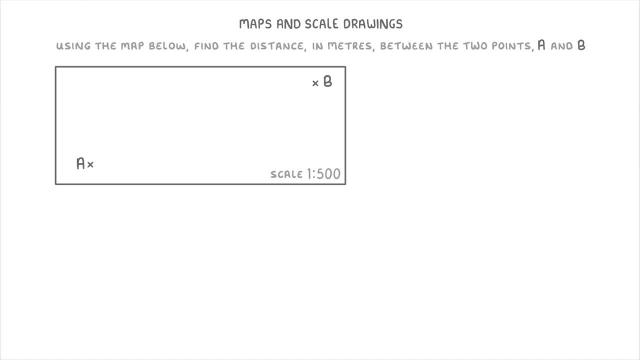 We're looking at our map to find the distance between the two points A and B And if we look at our map, we can see the two points they're talking about and we can also see the scale in the bottom right corner, which says 1 to 500, which means that our 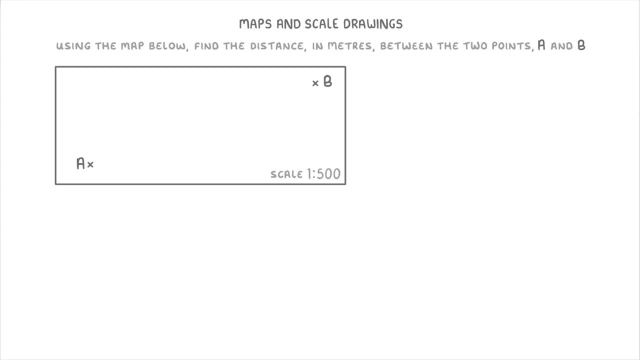 diagram is 500 times smaller than in real life. Now you don't have to do this, but what I like to do is change the 1 to 500, to 1 centimetre equals 500cm, because it means exactly the same thing, but it will be a bit easier to. 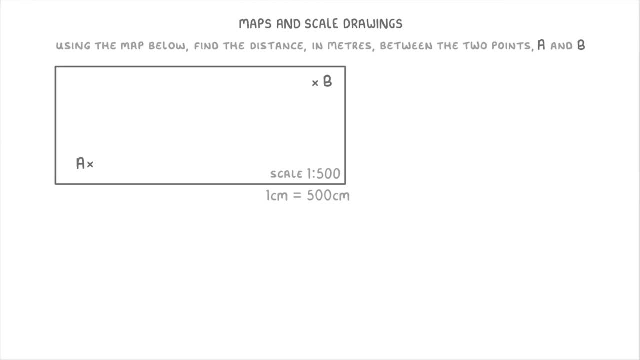 work with later. The next thing we're going to have to do is find the distance between A and B on our diagram, which we can do by measuring it with a ruler, and on my screen that's 9cm. Then, because we know from our scale that each 1cm on our diagram represents 500cm in real. 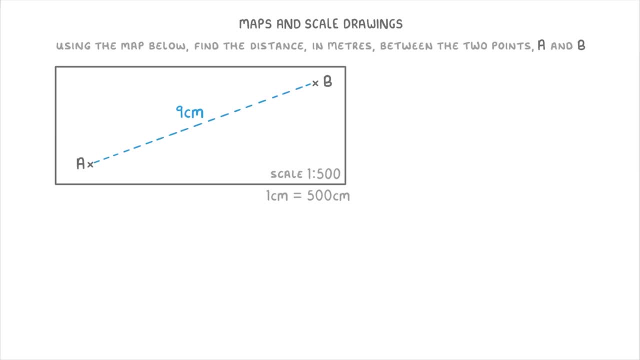 time we can work out what that 9cm must represent. So, because 9cm is 9 times bigger than 1cm, we also have to multiply the 500cm by 9, to get 4500cm. And then, to finish, all we need to do is convert that into metres by dividing it by 100, to. 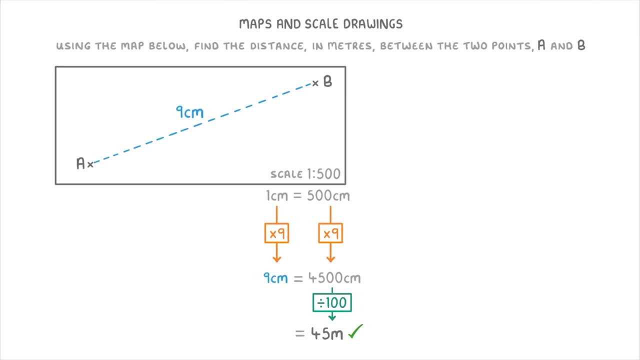 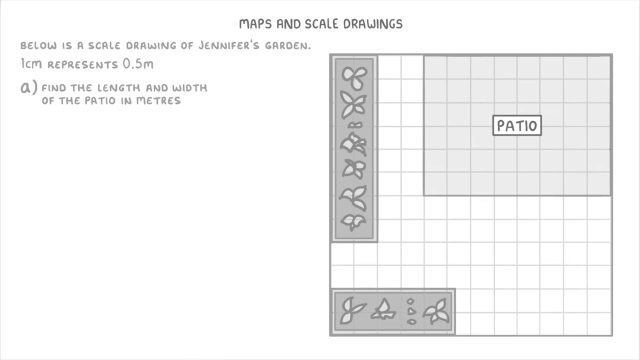 get 45m. So we now know that the point A and B are 45m. Okay, let's try a slightly different one this time. In this question we're told that the image below is a scale drawing of Jennifer's garden. 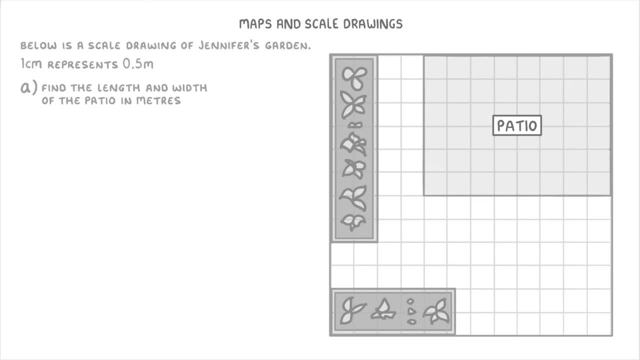 where each cm on the diagram represents 0.5m in the real world, And for part A, we're being asked to find the area of the patio in square metres. Now you might have noticed that they've done this drawing in a different way than in the. 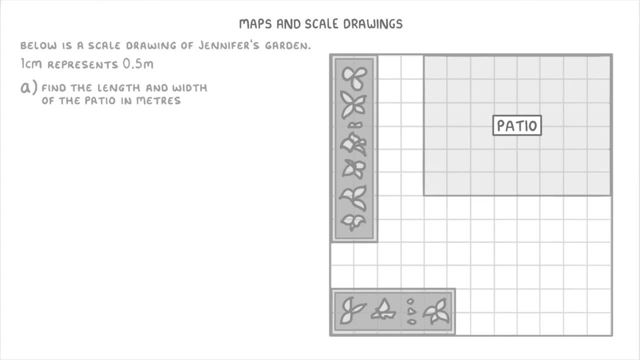 real world. They've done this drawing in a different way than in the real world. They've done this drawing in a different way than in the real world. They've done this drawing over a grid, And they actually do this quite a lot in exams, where each square is often 1cm by 1cm. 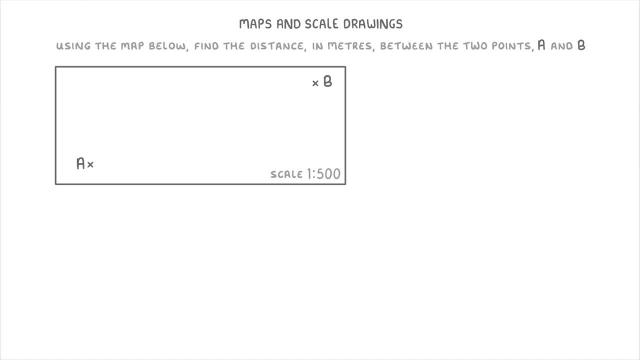 Now we're going to use the map to find the distance between the two points A and B, And if we look at our map, we can see the two points they're talking about and we can also see the scale in the bottom right corner, which says 1 to 500, which means that our 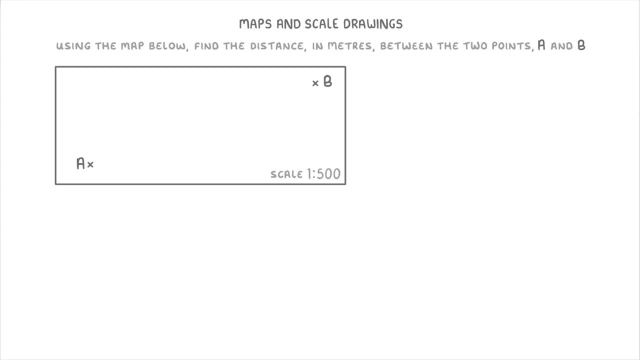 diagram is 500 times smaller than in real life. Now you don't have to do this, but what I like to do is change the 1 to 500 to 1 centimetre equals 500cm, because it means exactly the same thing, but it will be a bit easier to. 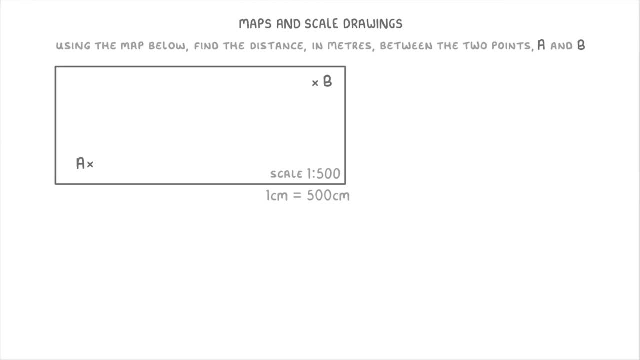 work with later. The next thing we're going to have to do is find the distance between A and B on our diagram, which we can do by measuring it with a ruler, and on my screen that's 9cm. Then, because we know from our scale that each 1cm on our diagram represents 500cm in real. 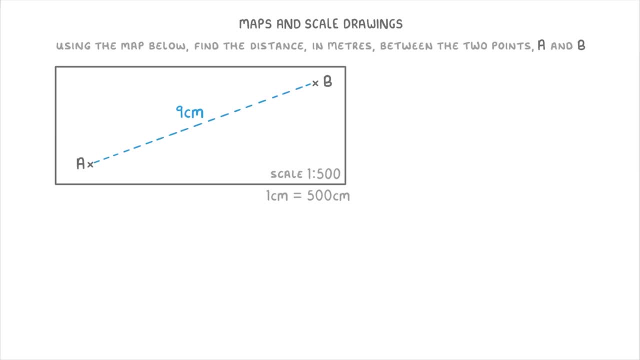 time we can work out what that 9cm must represent. So, because 9cm is 9 times bigger than 1cm, we also have to multiply the 500cm by 9, to get 4500cm. And then, to finish, all we need to do is convert that into metres by dividing it by 100, to. 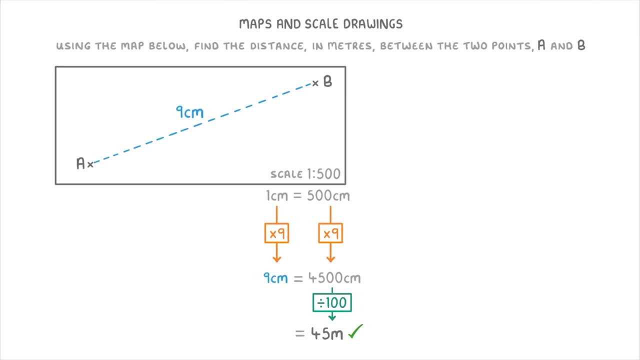 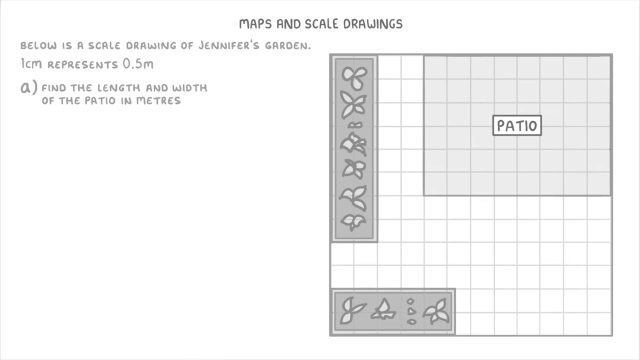 get 45m. So we now know that the point A and B are 45m. Okay, let's try a slightly different one this time. In this question we're told that the image below is a scale drawing of Jennifer's garden. 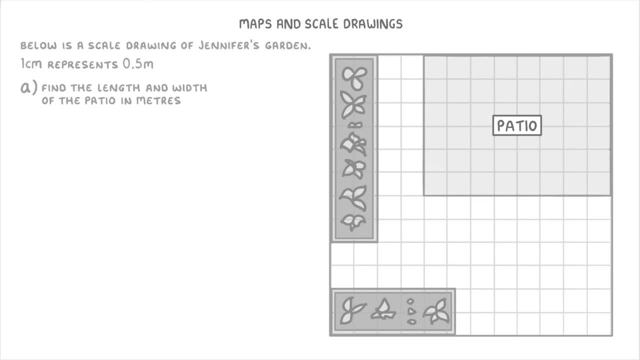 where each cm on the diagram represents 0.5m in the real world, And for part A, we're being asked to find the area of the patio in square metres. Now you might have noticed that they've done this drawing in a different way than in the. 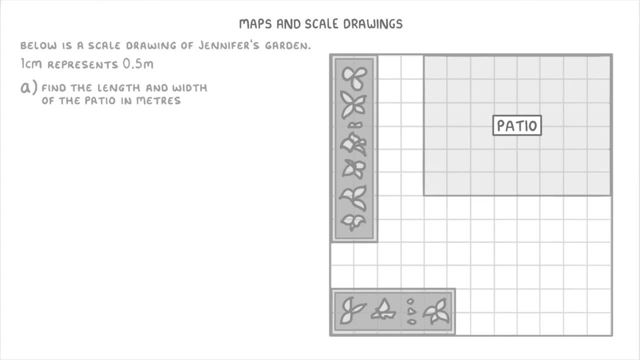 real world. They've done this drawing in a different way than in the real world. They've done this drawing in a different way than in the real world. They've done this drawing over a grid, And they actually do this quite a lot in exams, where each square is often 1cm by 1cm. 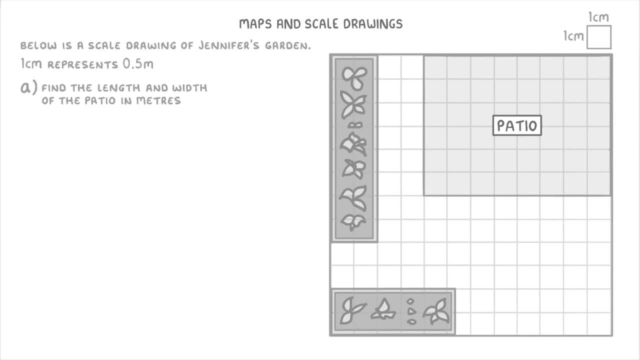 And this makes it easier for us to measure distances. However, the squares could also be different sizes, so it's always worth checking with a ruler. For this question, we'll assume that the squares are all 1cm by 1cm. 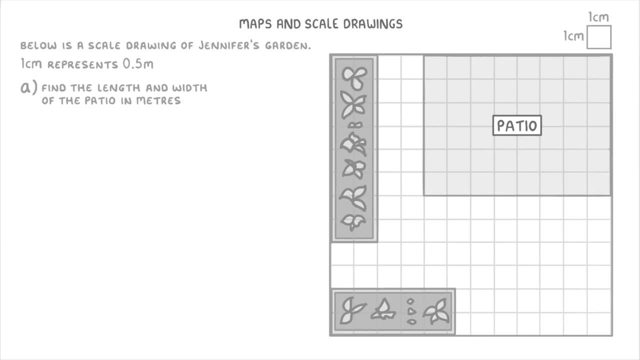 So, in order to find the area of the patio, we're first of all going to need to find the real length and real width, Because we'll then be able to multiply them together to get the area. To do this, we first need to measure how long they are on our diagram. 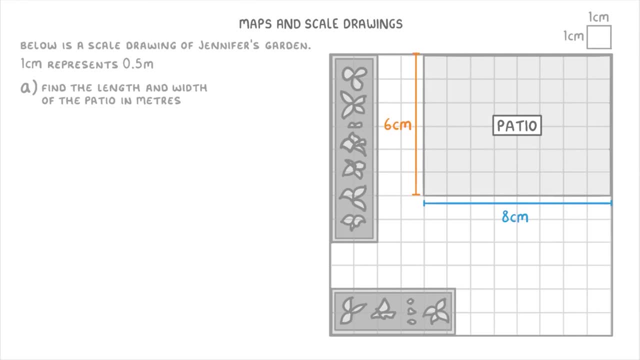 Which we can do using a ruler, which would give us 8cm and 6cm, Or by counting the squares, which would give us the same thing Because, remember, each square is 1cm. And now that we have these values from the drawing, we can convert them into real life. 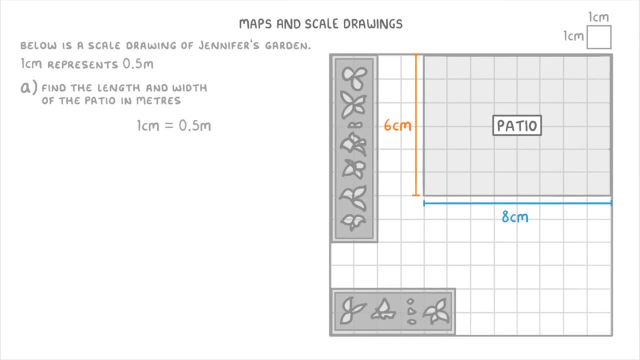 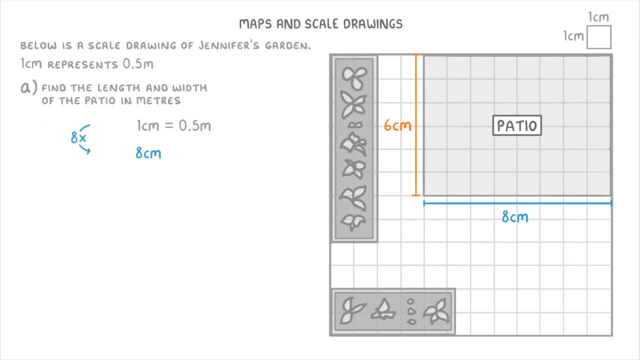 So because 1cm is equivalent to 0.5m, we can convert them into real life values. So because 1cm is equivalent to 0.5m, we can convert them into real life values. 8cm, which is 8 times larger, must be 4m. 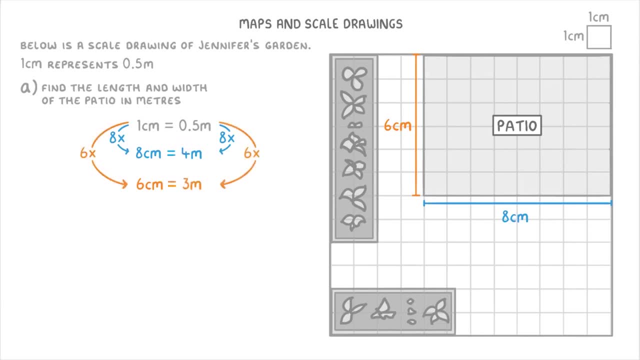 While 6cm, which is 6 times larger, must be 3m. So in real life, the patio area is 4m long and 3m wide. And lastly, because the area of a rectangle is equal to its length times its width, we 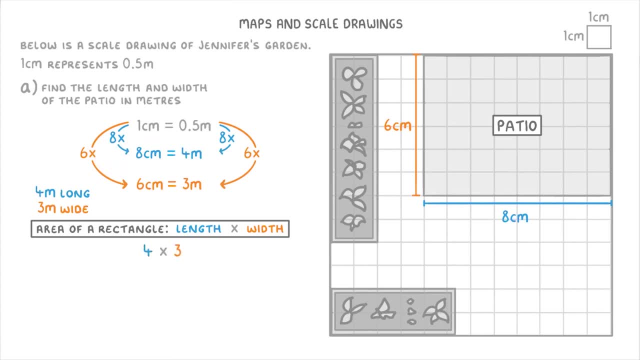 just do 4 times 3.. To find that the area of the patio is 12m2.. And finally, because the area of a rectangle is equal to its length times its width, we just do 4 times 3.. And lastly, because the area of a rectangle is equal to its length times its width, we 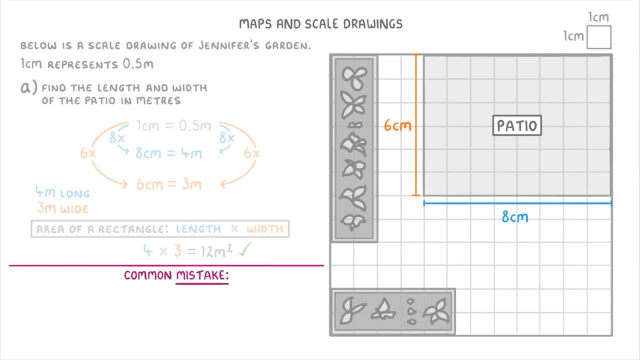 just do 4 times 3.. Now, one thing I want to point out here is that a common mistake with this type of question in exams is to find the area of the drawing in square cm and then try to convert that value straight to square m. 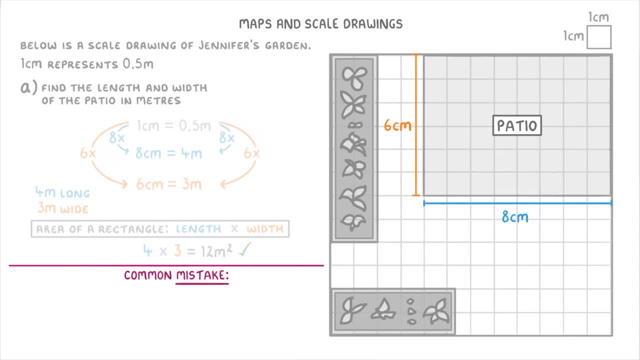 Which doesn't work. For example, if we found the area of the drawing by doing length 8cm times width 6cm, we can't XXX. We can't XXX it as well if we don't do it with the same square meters. 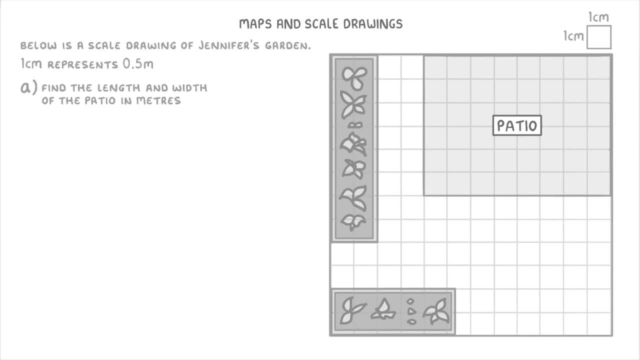 And this makes it easier for us to measure distances. However, the squares could also be different sizes, so it's always worth checking with a ruler. For this question, we'll assume that the squares are all 1cm by 1cm. 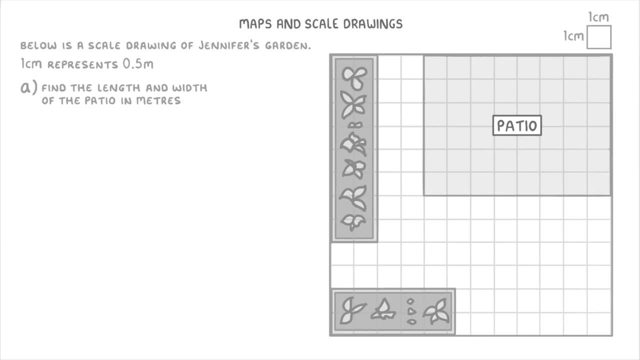 So, in order to find the area of the patio, we're first of all going to need to find the real length and real width, Because we'll then be able to multiply them together to get the area. To do this, we first need to measure how long they are on our diagram. 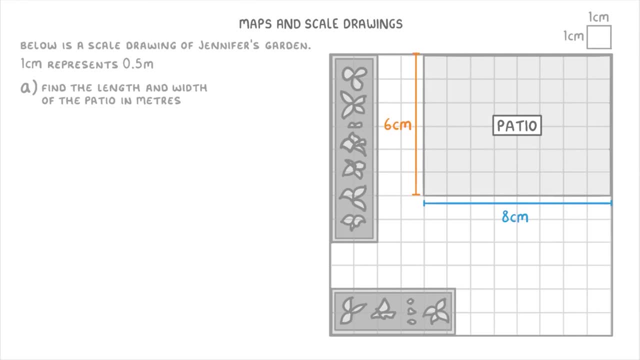 Which we can do using a ruler, which would give us 8cm and 6cm, Or by counting the squares, which would give us the same thing Because, remember, each square is 1cm. And now that we have these values from the drawing, we can convert them into real life. 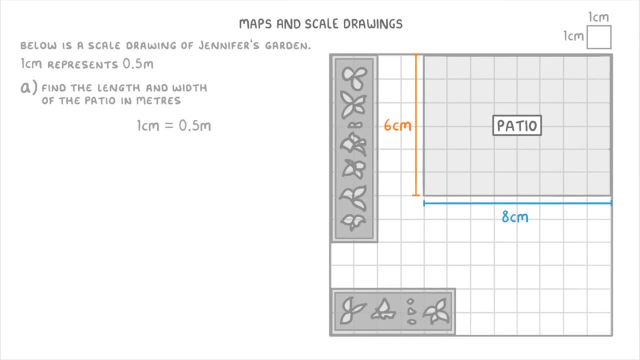 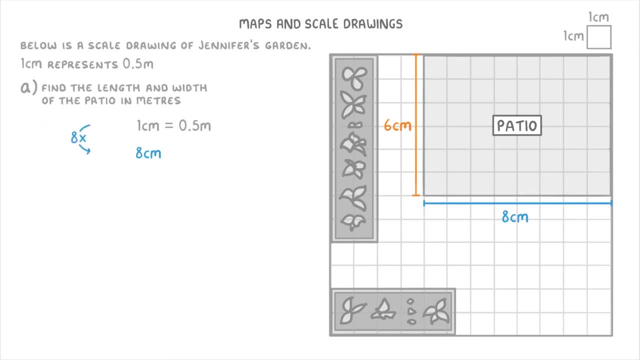 So because 1cm is equivalent to 0.5m, we can convert them into real life values. So because 1cm is equivalent to 0.5m, we can convert them into real life values. 8cm, which is 8 times larger, must be 4m. 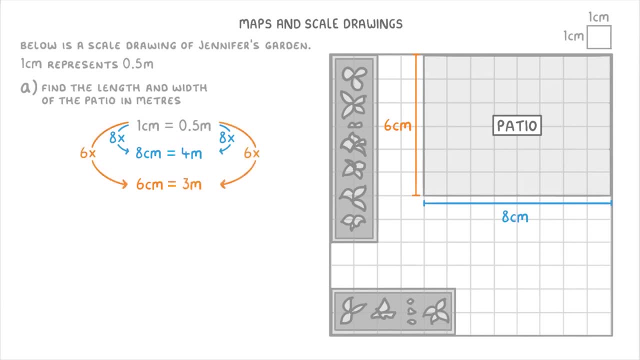 While 6cm, which is 6 times larger, must be 3m. So in real life, the patio area is 4m long and 3m wide. And lastly, because the area of a rectangle is equal to its length times its width, we 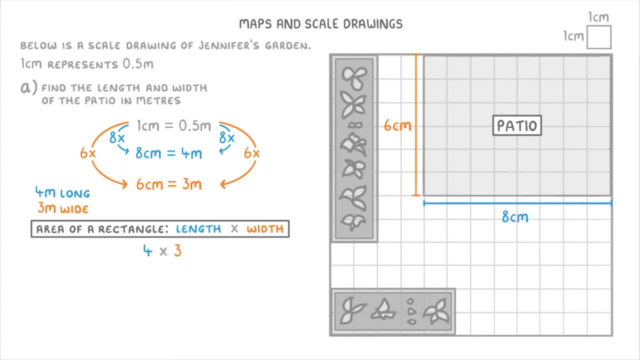 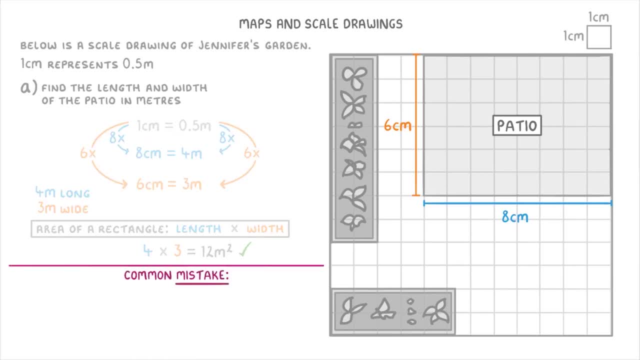 So because the area of the patio is 12m2.. Now, one thing I want to point out here is that a common mistake with this type of question in exams is to find the area of the drawing in square centimetres and then try to convert. 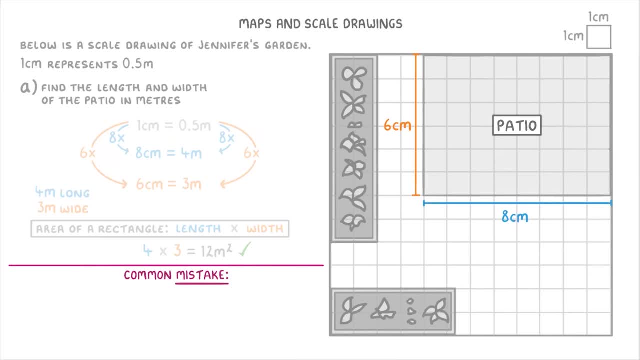 that value straight to square metres, Which unfortunately doesn't work. For example, if we found the area of the drawing by doing the length of 8cm times the width of 6cm to get 48cm2.. We couldn't then use our drawing to convert that value to square metres.